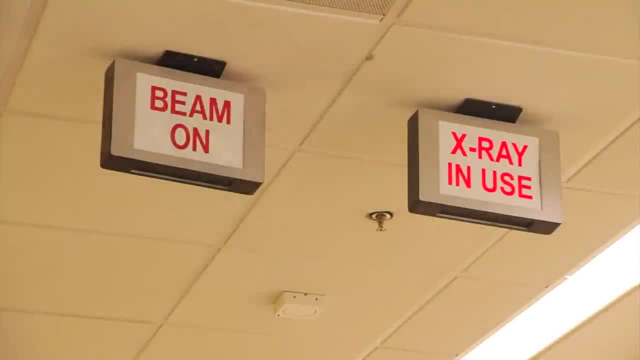 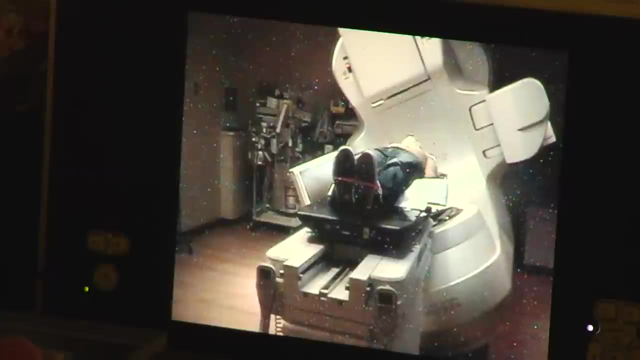 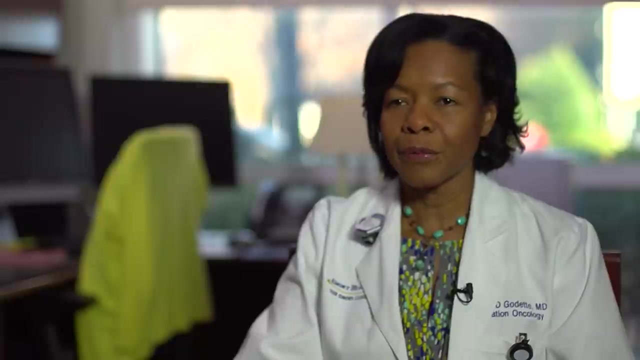 When x-rays are aimed at a tumor, it causes DNA damage that transform into tumors dying or having cell death. We treat many different types of cancers differently, with different forms of radiation. For prostate cancer, we may put radiation capsules into the prostate. 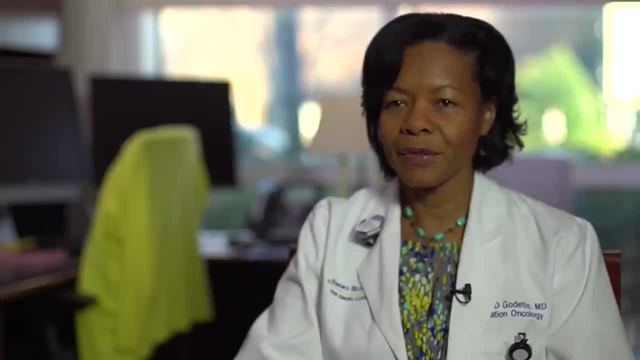 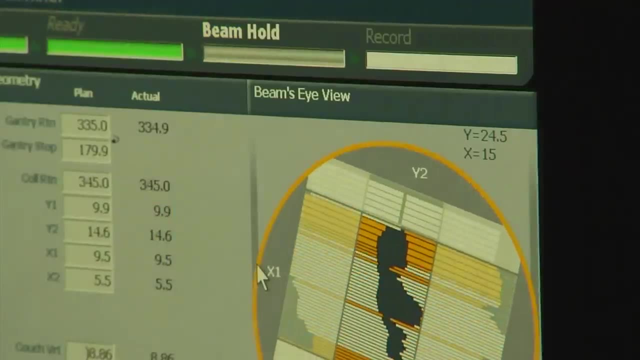 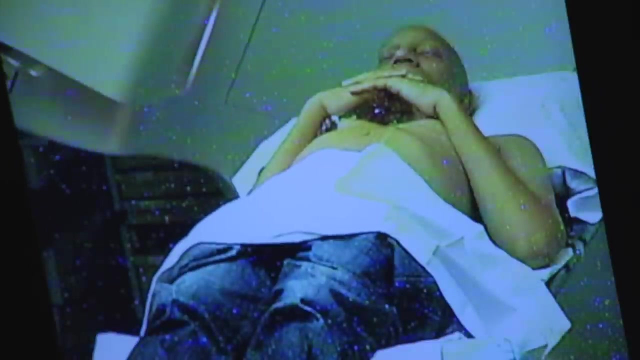 For breast cancer. we can now put a radioactive balloon in the breast or we can treat the breast from the outside. When we use external beam radiation today, we're using x-rays and we're focusing it in a three-dimensional, oftentimes four-dimensional way, because we can even control for the motion. 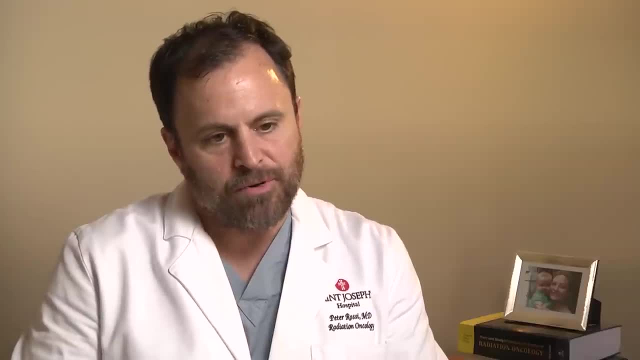 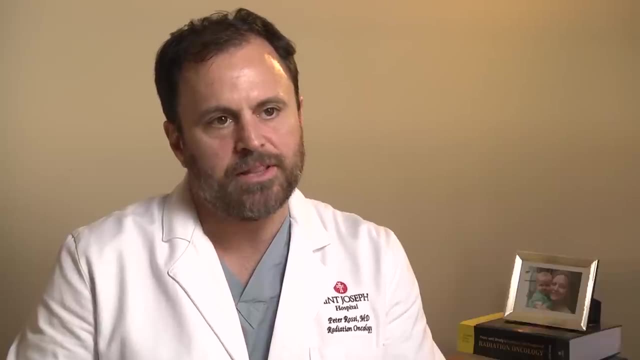 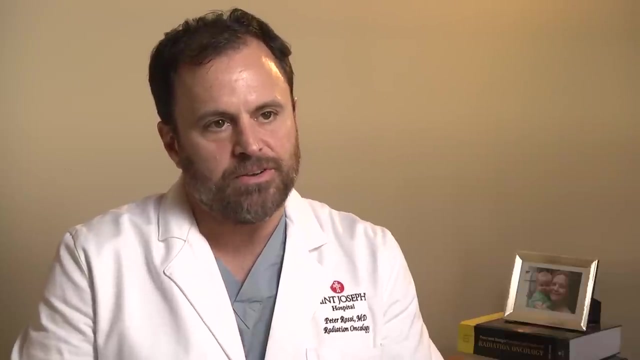 of breathing, the motion of the body. So it's topographically designed, very specific for every patient, and it has to do with where the tumor is in the body and what the organs are around it, and that leads us to having a treatment plan that is very unique and individualized. 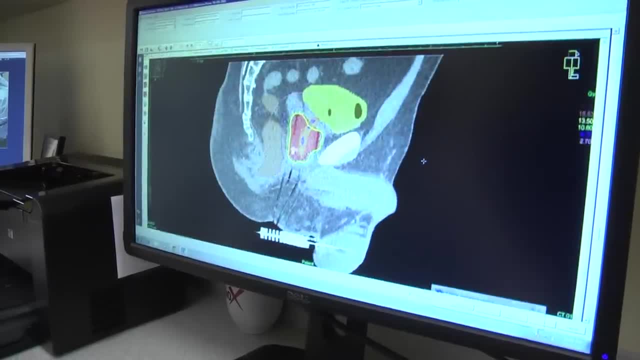 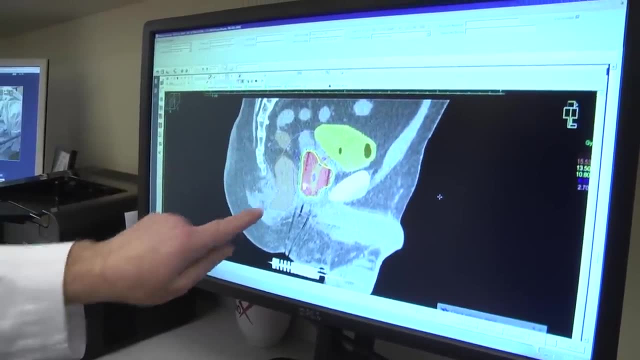 It's very precise and accurate. Internal radiation is a big part of radiation. In fact, historically that's how we started doing radiation. We knew if we could put radiation near a tumor or inside of a tumor we could have its greatest effect. 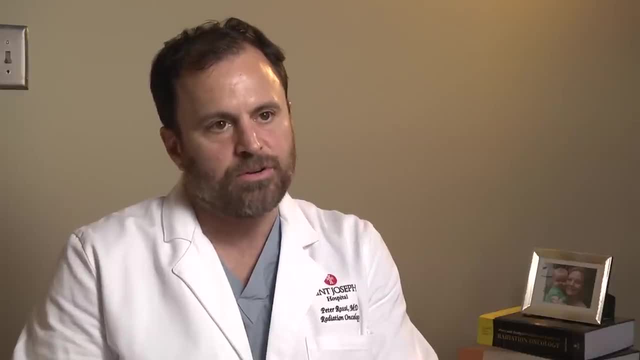 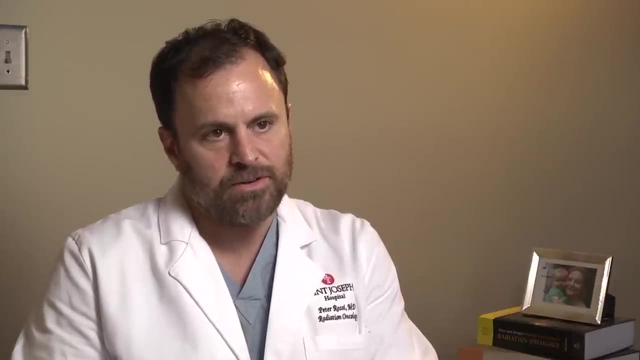 Radiation is delivered two different ways- what we would call low dose rate or high dose rate, and that's just a difference in the strength of the radiation seed or the source that we're using. When we use radiation, it's usually directed at a very high dose rate. 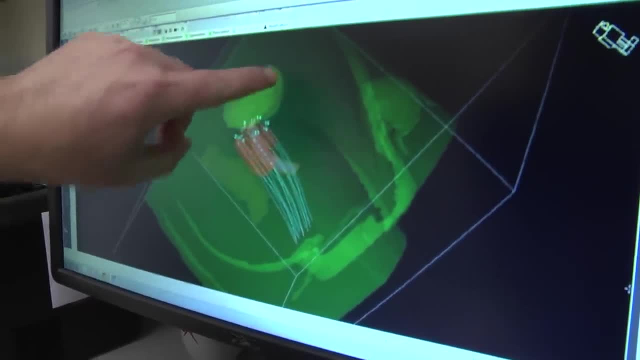 It's usually directed at a very high dose rate and that's just a difference in the strength of the radiation seed or the source that we're using. So it's a very specific area of the body and the side effects relate to that area of. 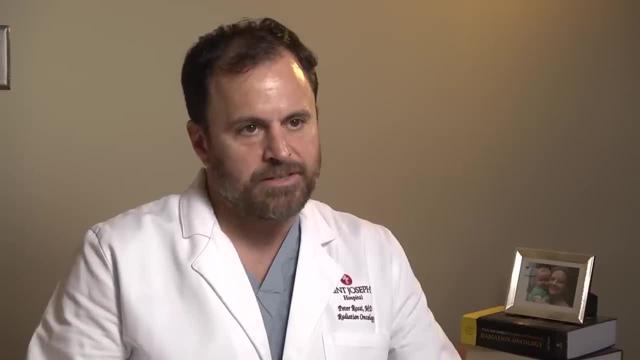 the body. Some people experience no side effects with radiotherapy and that's not necessarily uncommon. but we prepare you for even the worst case scenarios because there are very rare side effects that radiation can cause as well, But it is very specific to the body. 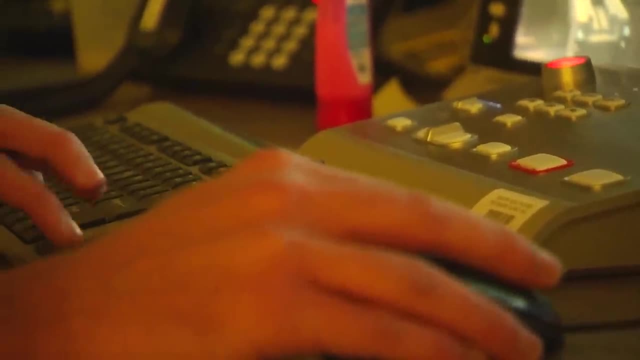 Within the last 10 years it has advanced tremendously. We've become a lot more computerized. We need to be more preventative, We need to be more efficient, We need to be moreึ, We need to be more effective, We need to be more skillful.